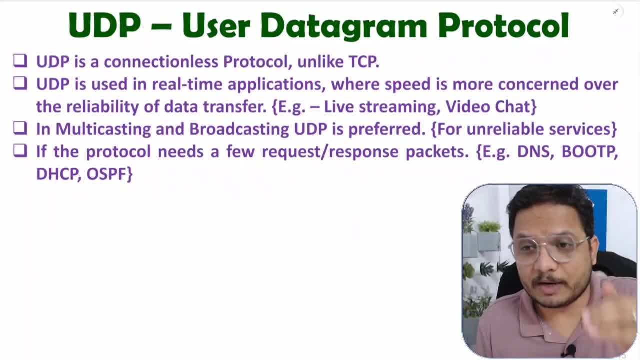 know first why UDP is preferred in computer network. See: UDP is connectionless protocol, unlike TCP. We have already seen TCP in great detail. In TCP we have three stages: Connection establishment, data transfer and connection termination. So for connection establishment, 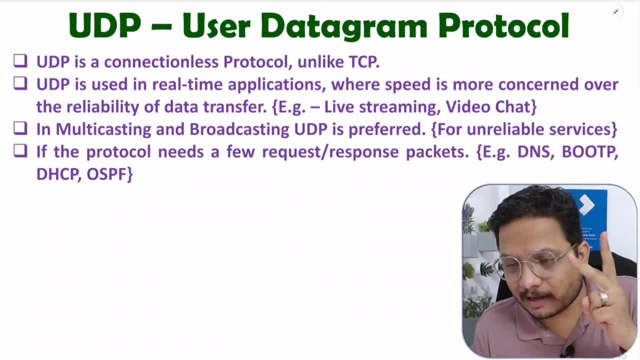 you need to have some time. Then you will be forwarding data. That data forwarding will be reliable data forwarding. And in connection termination, we will be terminating connection in between source and destination. But in UDP we don't need to establish connection. 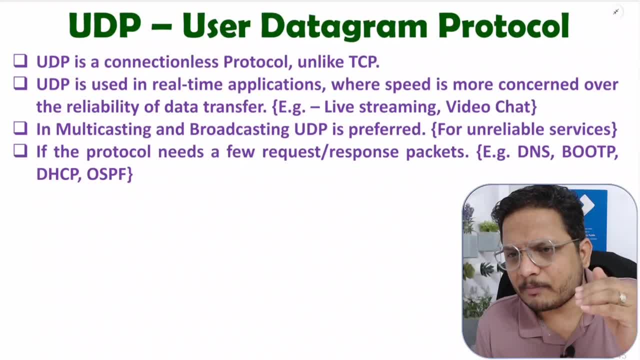 That's why you will be saving some time. So here see, UDP is used for real time applications. So in real time applications you don't have time for connection establishment, data transfer and connection termination. So that's why in real time applications we use UDP In. 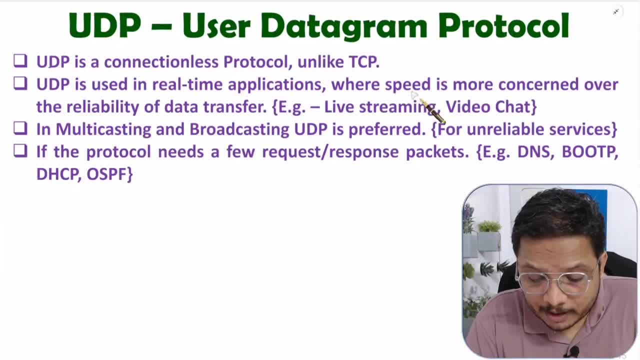 real time applications. we prefer more speed over reliability, As if you want to have reliable data transfer, As if you want to forward video file, then you should prefer TCP, in which you will be forwarding data with reliable service, where there will be no data loss, But as if you. 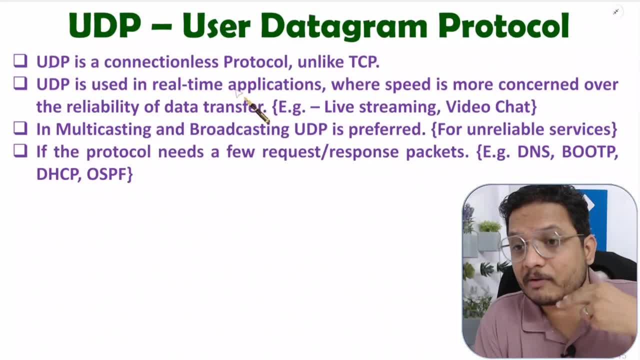 talk about real time applications like video chat. So in that situation you will be using UDP, in which speed is more concerned. We are not concerned about reliability. If some data are missing, then also that is fine in UDP, Right, As if you have real time. 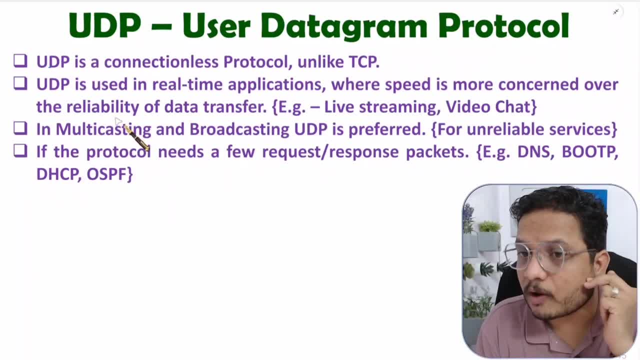 application. So you should know, see, as if you want to forward file, at that time you should be using TCP. But for real time application, like live streaming video chat, you will be using UDP. Why? The reason is: in video chat, if some data are missing, then 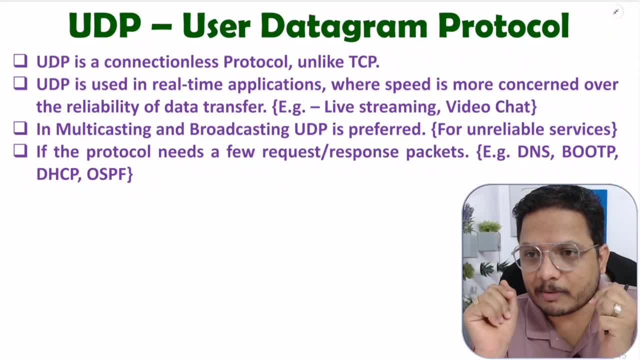 also. it is fine, But application should be real time. If you have connection oriented service like TCP, in that situation, what will happen? There will be more time for buffering, It will consume more time And because of buffering and delay, TCP is not preferred. 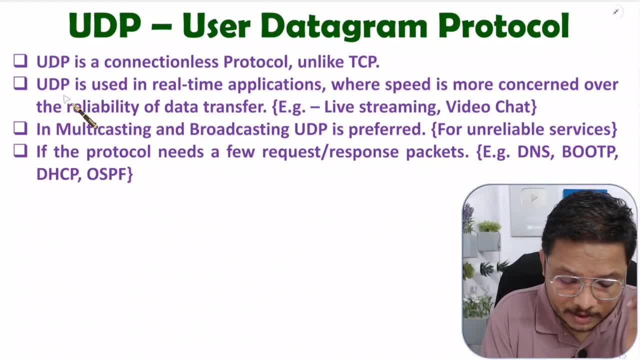 in real time applications, Right. So UDP is used for real time applications where speed is more concerned over reliability- See in multicasting and broadcasting. also, UDP is preferred. Now you might be thinking like, why should we have UDP over TCP for multicasting? 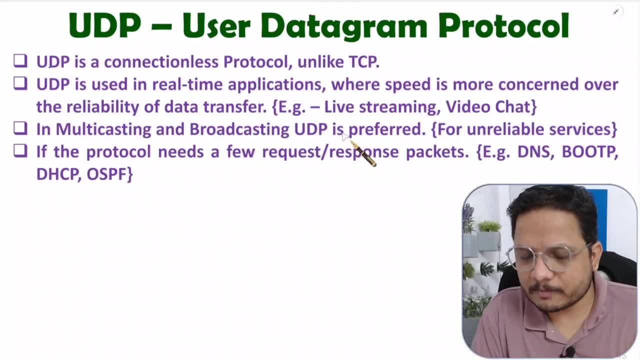 and broadcasting. So let me explain you that by watching this video. one practical analogy: Here you see, we are having one sender. In multicasting and broadcasting we will be having multiple receivers. So let us say receiver R1, R2, R3, R4. that is how multiple 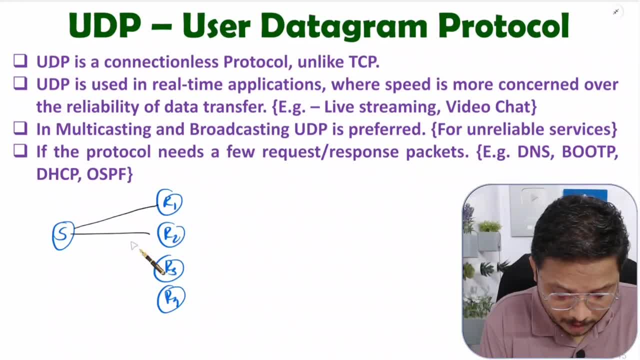 receivers are connected over here, right for broadcasting and multicasting. Now see, what will happen is, in case of TCP, there will be sender window and receiver window. So receiver is having window over here. So with receiver it is fine, there will be single window. But with TCP sender, 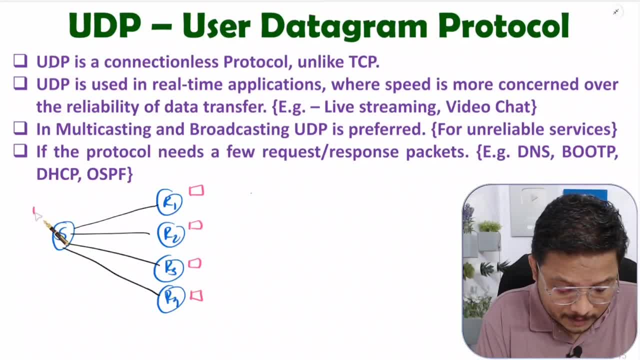 will be having separate window for all the receiver. So here I am showing you four different windows for four receivers. But if you talk about practical scenario, like in broadcasting, let us assume you want to broadcast message to hundred receivers, So with hundred receivers you need to. 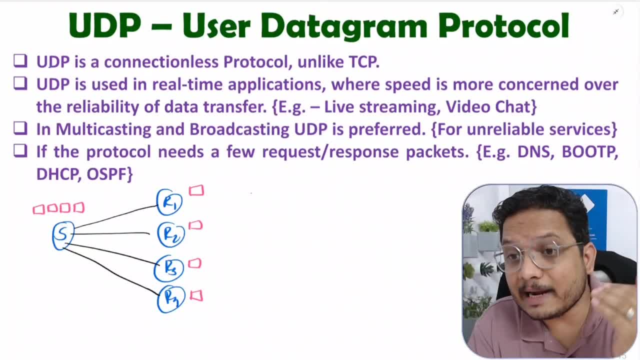 have hundred windows over here, Hundred slash sliding windows with TCP. So at that time the sender requires humongous computational complexity, Like CPU should be very powerful at sender, as if sender is broadcasting message to hundred people. Why the reason is you need to have hundred sliding windows. So that's why, see, TCP is not preferred. 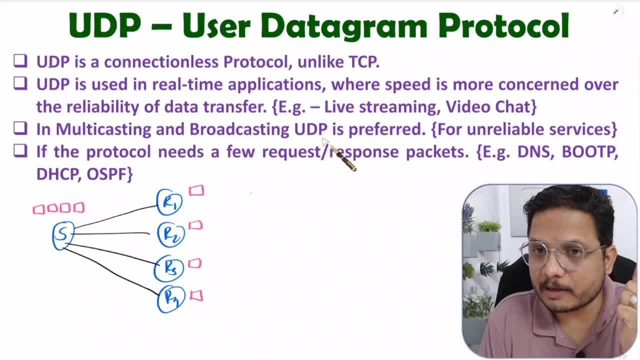 for multicasting and broadcasting. Here we should prefer UDP, where we will be having unreliable service right See for unreliable broadcasting and multicasting, only UDP should prefer. If you wanted to have reliable multicasting and broadcasting, then you should go for TCP. But in that 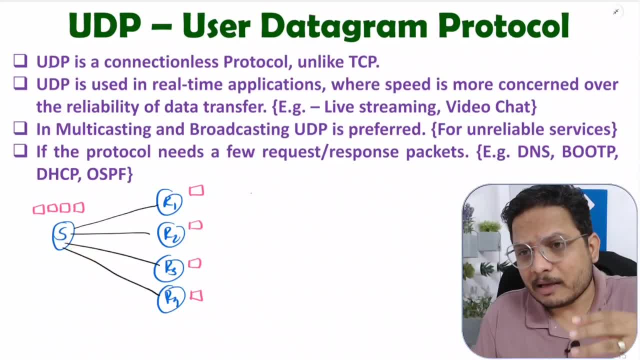 this sender will be having higher complexity in terms of CPU. There will be more memory in terms of RAM or data access Right. So that is highly required in case of broadcasting and multicasting Right. See, if protocol needs few request and response packets, then also UDP is preferred, Like you see in TCP, for connection. 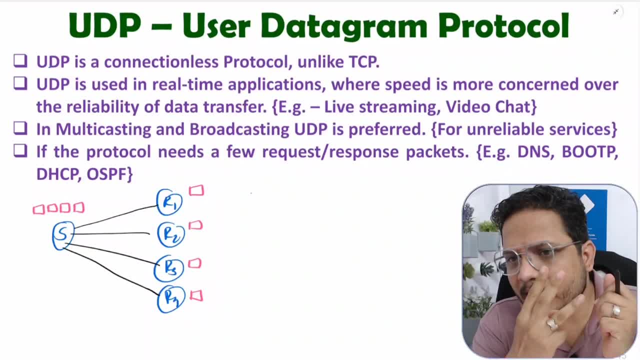 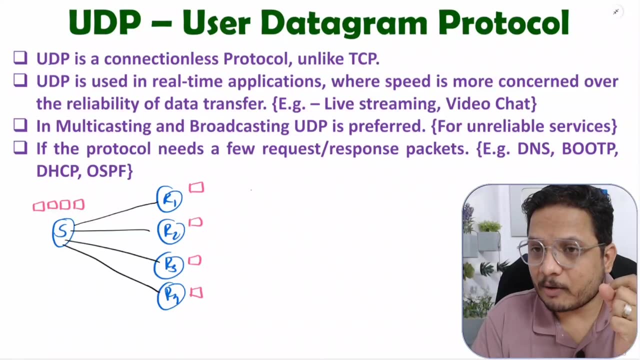 establishment. there will be three-way handshake. There will be three-way handshake, So those three-way handshake will make sure there is connection establishment. Then after there will be data transfer Right. But if the protocol that needs few request and response packet, Like we have already seen, 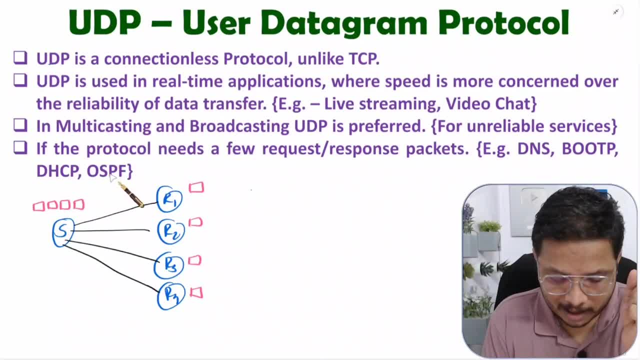 How would be? is there about DHCP protocol is there? How routing protocol like OSPF is there? So in that we just need to have few packets only. You don't need to establish connection like three-way handshake every day. So in that situation we don't prefer TCP. Now you might be thinking like how you can? 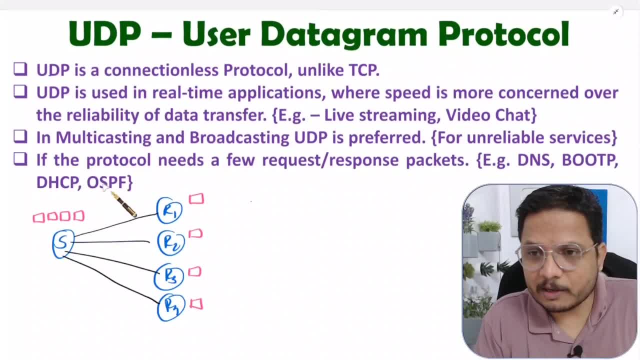 say this: this protocols uses UDP. I'm not saying this, protocols are using UDP. What I'm saying is it is accessing computer network as per UDP. Inherently, these protocols are accessing computer network as per UDP. See, in UDP we don't provide connection establishment and in TCP we need. 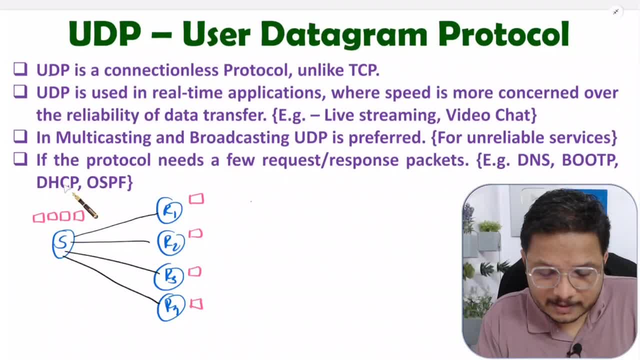 to have connection establishment. So for BOOTP, for DHCP, do you think like you are providing connection establishment and then after you are accessing internet, No, Practically when you turn on your computer, on computer network and when you see how many packets that we 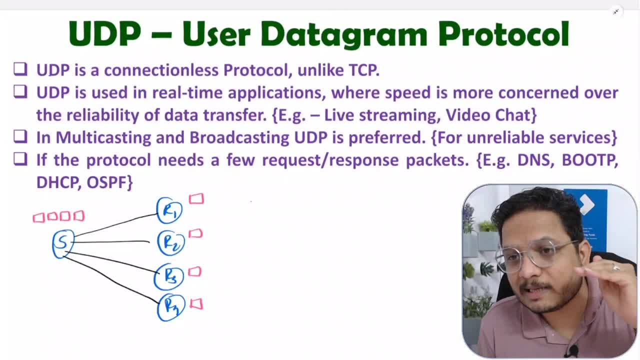 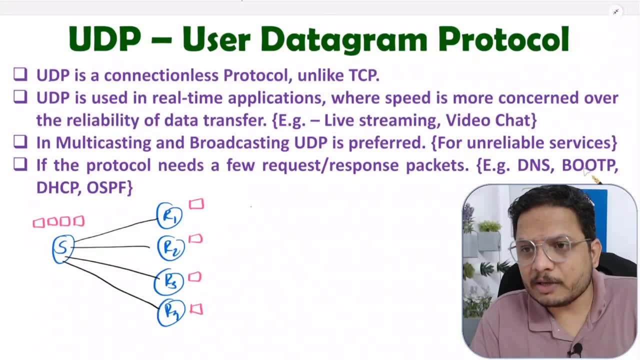 are receiving. so in that when you talk about TCP, data transfer, so before data transfer we were been having connection establishment. But in case of BOOTP you just need to have few request and response packets. You don't need to have 3 packets for connection establishment. 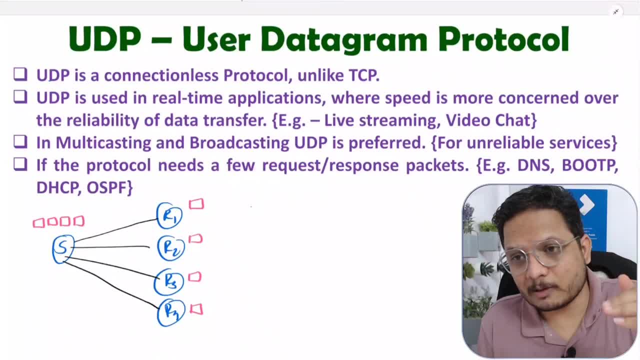 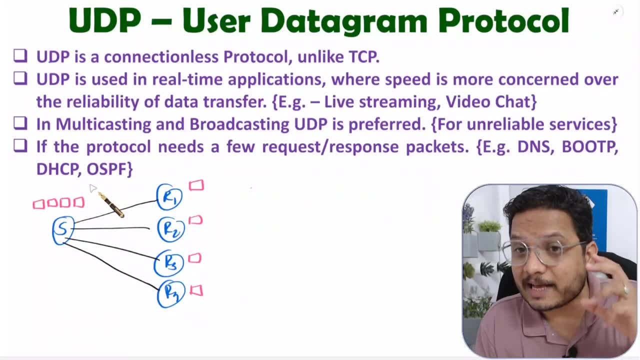 If you have. in that case your services will be very slow. So inherently you can say that these protocols are using services as per UDP Right. So, in short, all you can understand is TCP. that is, reliable service in which there will be no data loss If some data is missing. 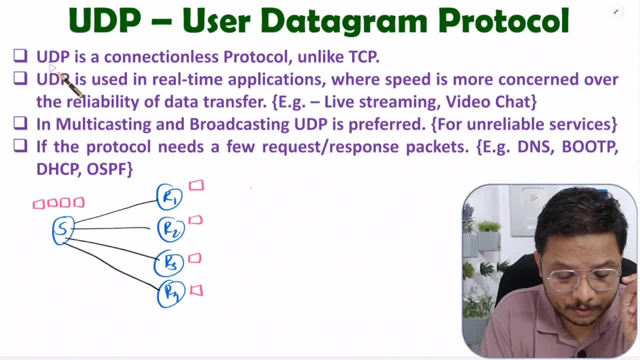 in that case there will be retransmission. In case of UDP, we are having connectionless protocol. You don't provide connection establishment and all those stuff Here you will be more concerned towards TCP. You don't provide connection establishment and all those stuff Here you will be more concerned towards TCP.